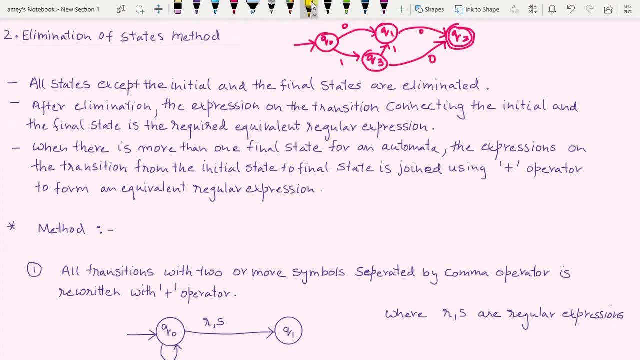 what we are going to do is these intermediate states, like, for example, q1, q3, all these intermediate states will be eliminated. So, finally, what will remain is only the state q0, which is initial state, Then the final state, say q2, and in this particular process, in this particular method of elimination, 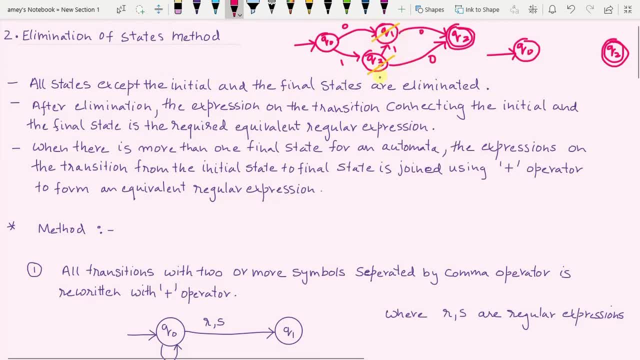 of states, all the intermediate states which are there in the automata. they will be eliminated. And finally, you will see that the regular expression that is required will appear on the transition that connects the initial state and the goal state. So you will find the regular expression on the transition line that connects the initial 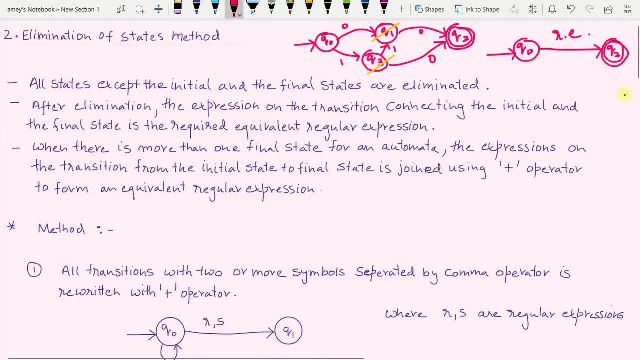 state and the goal state. It can so happen that there are more than one final state. suppose qn was another final state. Then again, all other intermediate states connecting q0 and qn, all of those will be eliminated and the regular expression in this case will be: on the transition line connecting q0 and. 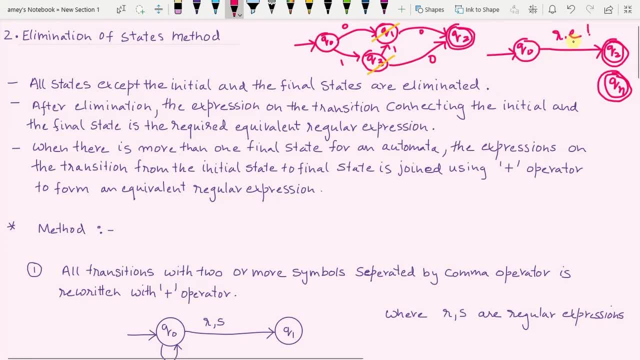 q2, you will get one regular expression, S. Similarly, on a transition line connecting Q0 and Qn, you will get second regular expression. So the final regular expression will be what It will be: Re1 or Re2.. So either you will get this or you will get this. 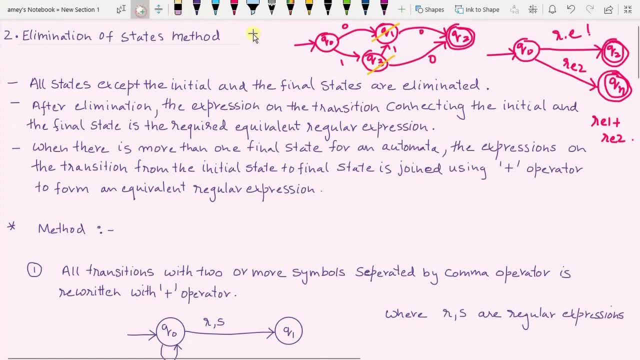 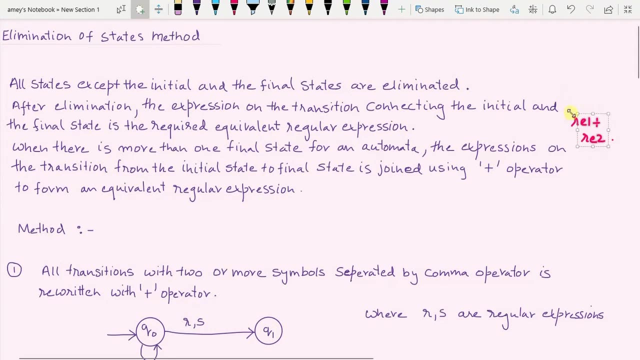 So this is basically the idea of elimination of states method that we are going to see today. Okay, Okay, Okay, Okay, Okay, Start recording from here. So all the states, except the initial state and the final states, all other states shall be eliminated. 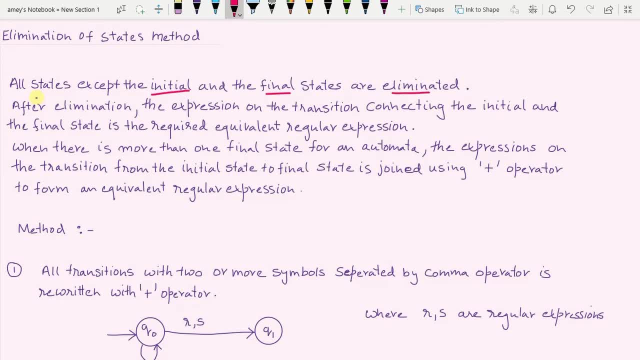 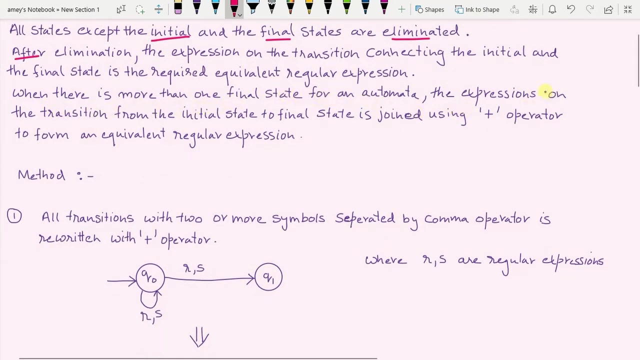 So this is the first thing that I have just spoken about. Second, after elimination, what will happen? The expression on the transition connecting this initial state, Connecting this initial state and the final state, is the required equivalent regular expression And, as I have already said, when there is more than one final state for an automata, the expressions: 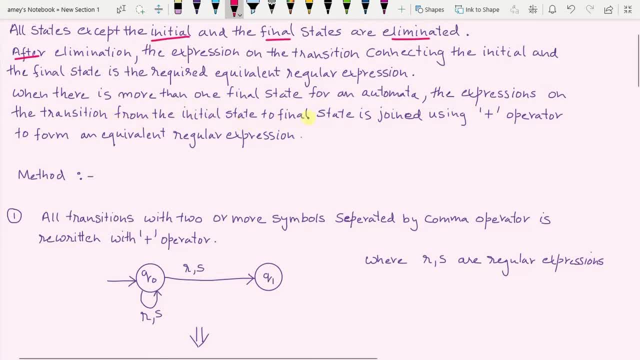 on the transition from the initial state to the final states. all these small, small regular expressions connecting initial state and each of the final state, all of them will be joined using plus operator to form an equivalent regular expression. Okay, Now to do this- elimination of states- there is one method. 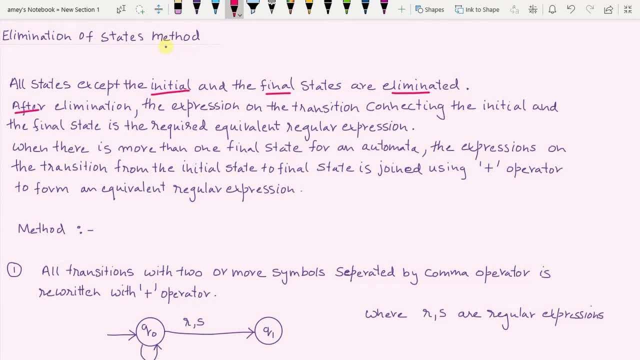 And basically a student is going to work based on the observations. We will have to observe the automata, see what are the components of the automata at that particular instance and apply one of these. I am going to show you some rules, Okay. 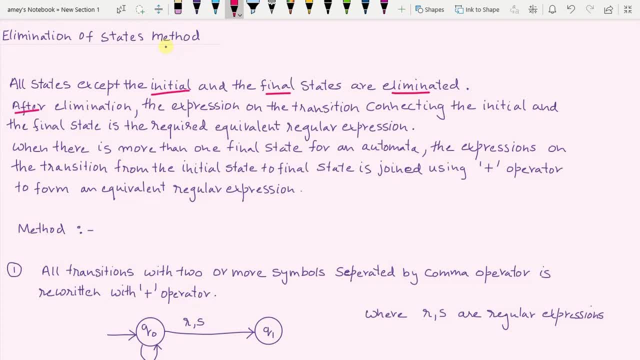 How to eliminate a particular state when there is this particular case or the other particular case. So for each case there are different rules that you have to apply. So you have to analyze the problem as you go. Okay, So you have to analyze the problem, analyze the automata in this whole process and based 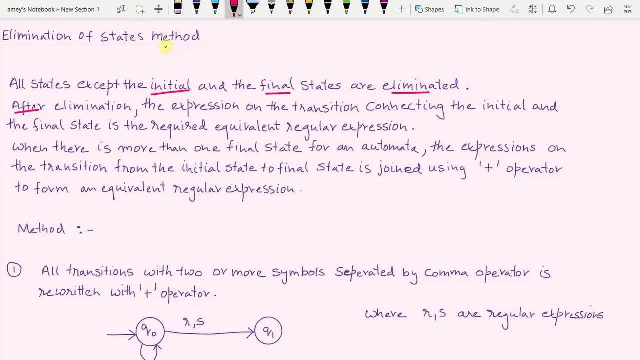 on your analysis. you need to go on eliminating the states. Finally, you should stop when you have only two states, that is, initial state and the final state, or if there are multiple final states, then the automata should have only initial state and all those final states and the regular expression appear on the transition line connecting. 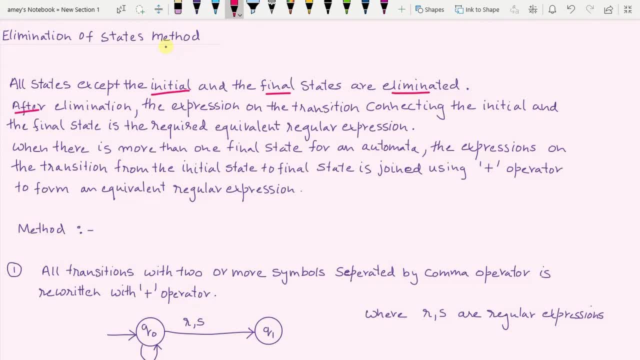 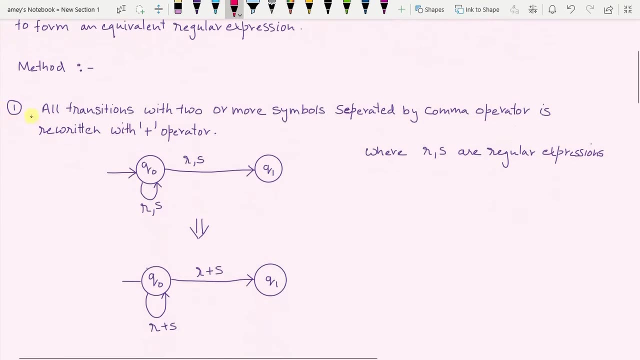 this particular input. Okay, So you have to start state and each of the final state, and if there are multiple final states, there will be plus symbol connecting each of the regular expression. We shall see this as we solve. Now let us see the first rule. 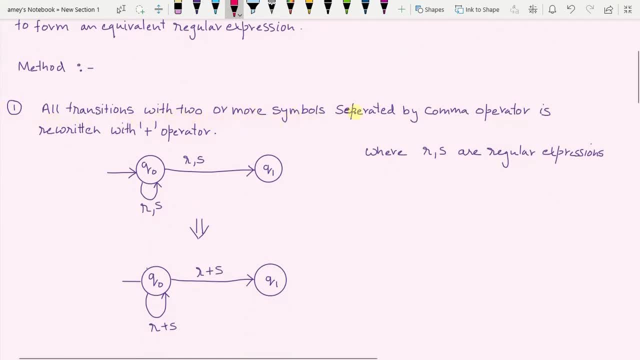 Okay, All the transitions with two or more symbols separated by a comma operator is rewritten with plus operator. Now, many a times we see in a given automata, many a times there is a comma that appears. For example, this means from state q1, sorry, from state q0. on reading r, you go to q0 and 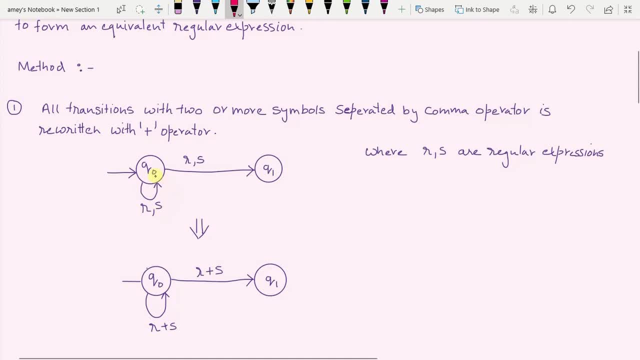 from the same state q0 on reading s also, you go to q0. So whenever you have two input symbols on reading, two different input symbols, the same transition happening, you connect it with comma. We have seen this earlier right. So this comma means from q0 on reading r, you go to q0. 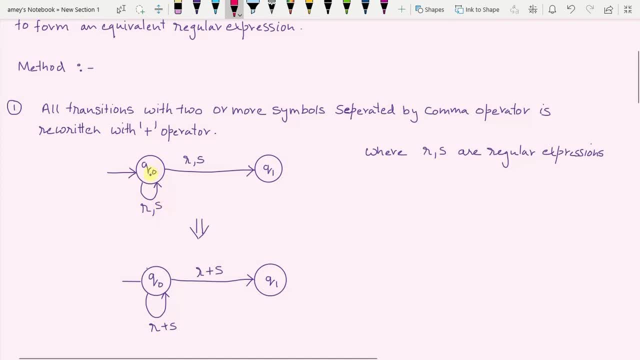 Comma means or From s also, Okay, I mean from q0. on reading s also, you go to q0.. So either when r is encountered as input symbol or when s is encountered as input symbol from q0, the transition remains same: it goes to q0 itself. that is the meaning of comma. 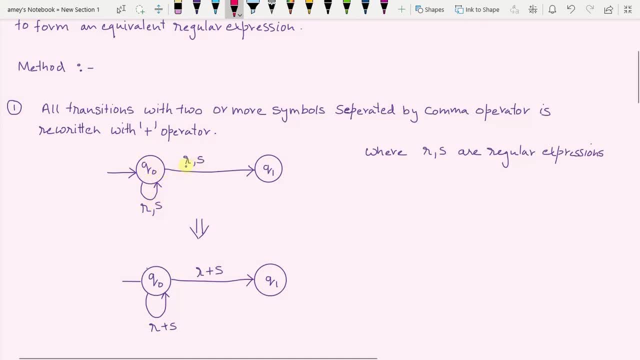 Similarly, when comma appears here, it simply means that from q0 on reading r, you go to q1, and also, or you can say: or from q0 on reading s, also, you go to q1.. So whether it is r or reading s, That is r or s which is read from q0, you are always able to go to q1, okay. 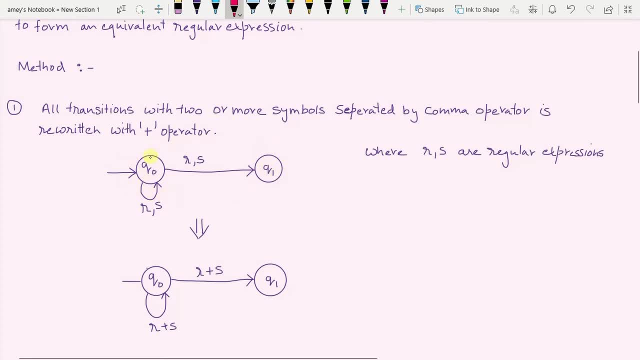 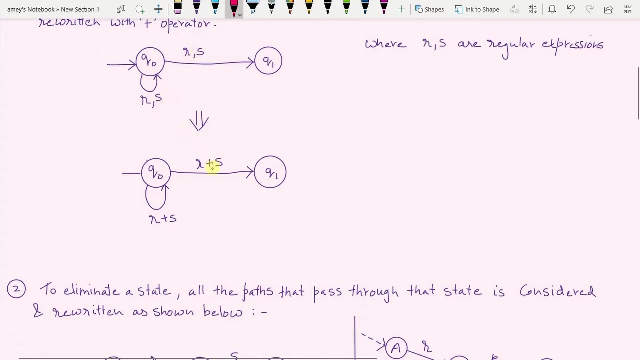 So suppose this is the automata that we have, where of course, r and s are the regular expressions, then this comma. first thing: whenever there is comma, okay, comma has to be replaced with plus. So what I have done: wherever there is comma, that is here and here the comma has been replaced. 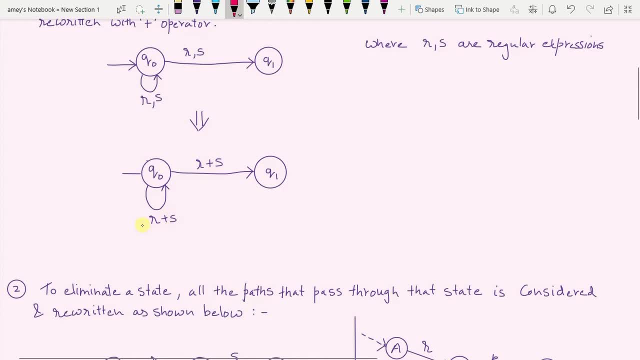 with plus and plus. okay, Because we have already seen a rule and the rule says that if there is a comma, that is, a coordinate system, Whenever in a finite automata or whenever in the regular language there is comma, an equivalent regular expression, In that what will happen? comma will be replaced with plus. okay. 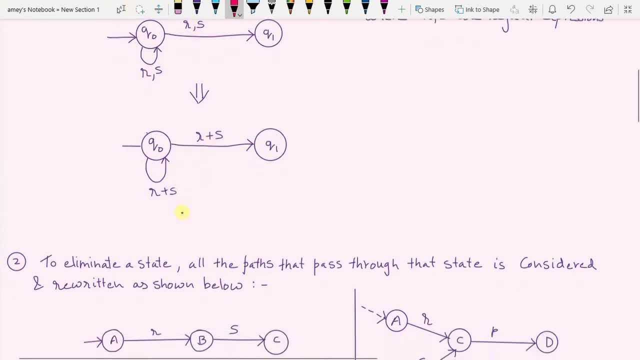 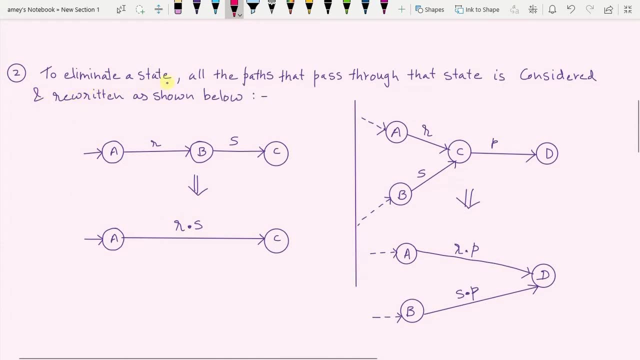 So wherever there is comma, you need to replace comma with plus. Now let's go for the rule 2. now the second rule to eliminate a state. So in this rule we are going to see how to eliminate a state, how to remove a state. 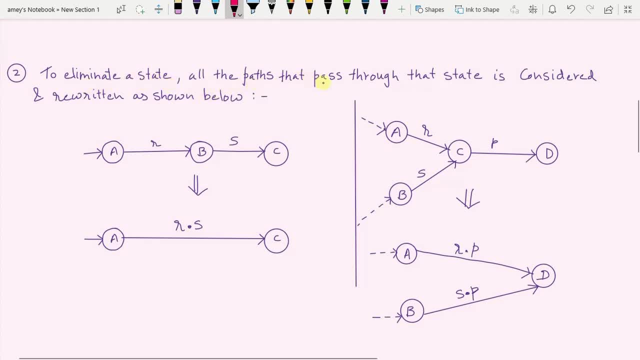 So to eliminate a state, All the parts that pass through the state are removed. Now let's recover the state through. that state is considered and rewritten as shown below. okay, now you have to be very careful here. now just see, from state A you go to B, and then from state B you go to C. 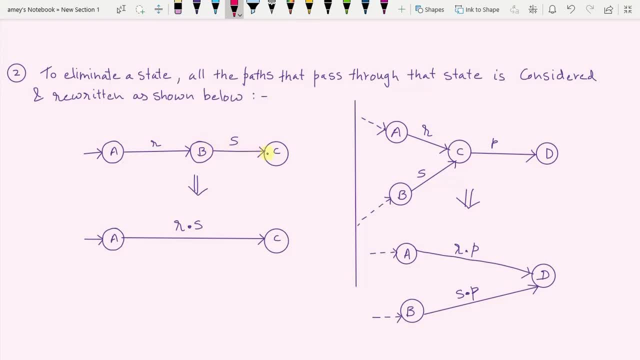 right, from A you go to B, and then from B you go to C, and now suppose you want to eliminate the intermediate state B. okay, suppose you want to eliminate the intermediate state B. this B has to be eliminated. so now you should think this way: now, from A on reading R, you 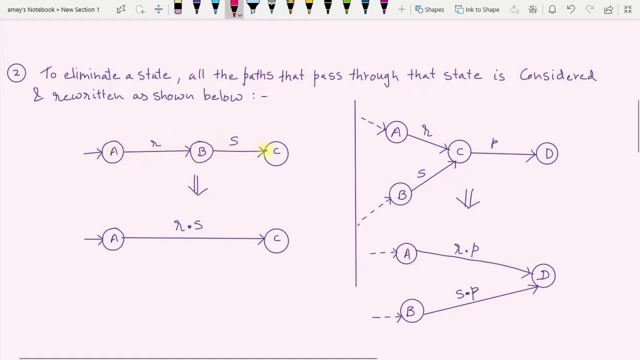 are going to B. from B on reading S you go to C. so how A and C is connected? A and C are indirectly connected. so it simply means that from A after reading R and then after R reading S, so when R is read and then after that when S is read, then you go to C. so A is indirectly. 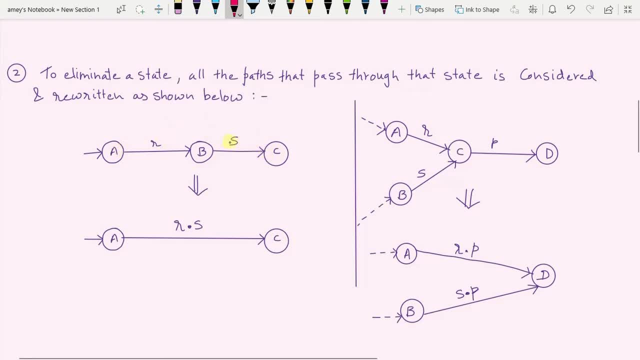 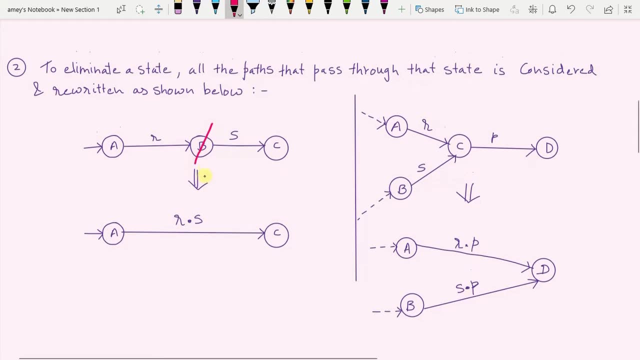 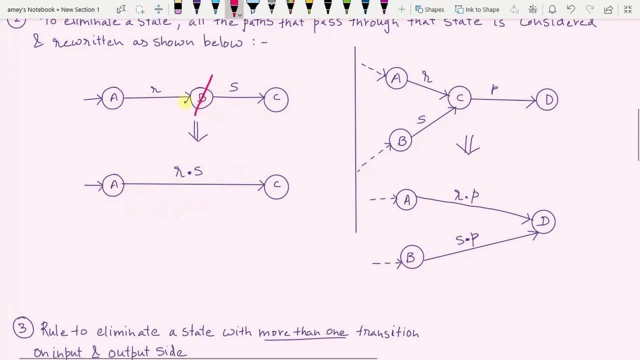 connected to C through R S as input, R dot S as input. so now, when B is supposed to be eliminated, if I want to eliminate this B, okay, then what will happen? A and C will be directly connected through one transition, and R and S, these two inputs, will be returned together. 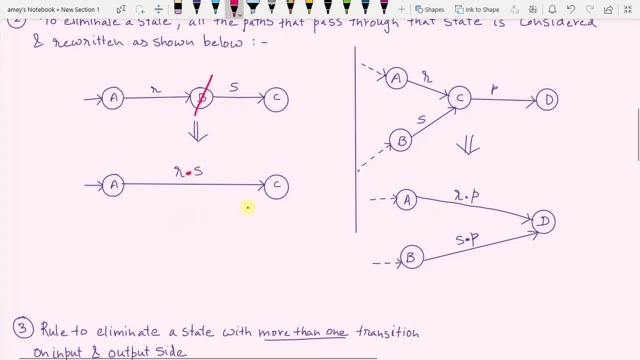 with R, dot S, so you will use dot operator. that is the meaning of it. okay, now the second thing. Suppose It is this type. now, this is simple. this particular case is very simple. but let us look at this particular case now. my aim is suppose I want to eliminate this C. okay, I want to eliminate. 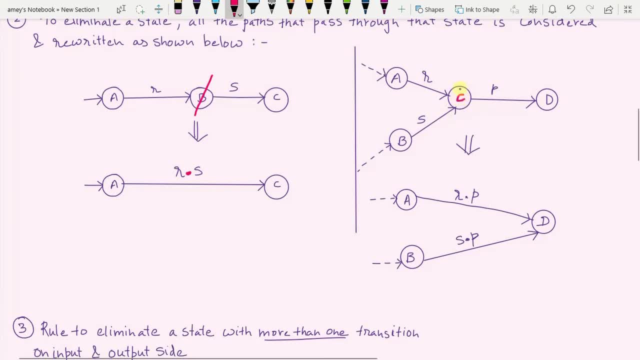 this particular C now to eliminate C. I cannot simply eliminate C. there are certain things that you need to see now. just see: A is connected indirectly to D. A is connected indirectly to D through C. okay, So if I want to remove this C, okay, then I will have to show a transition: direct connection. 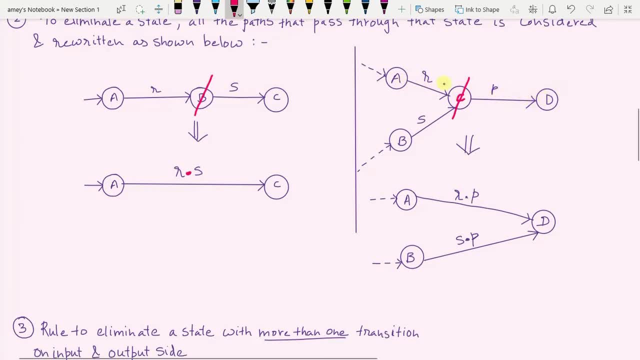 from A to D and the input that will appear on the transition will be R dot P. okay, this will be the input. Similarly, when I want to eliminate this intermediate state, then I will have to have a transition that directly connects B and D. okay, Okay. 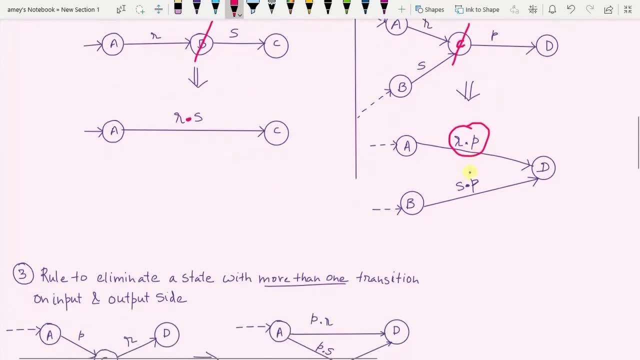 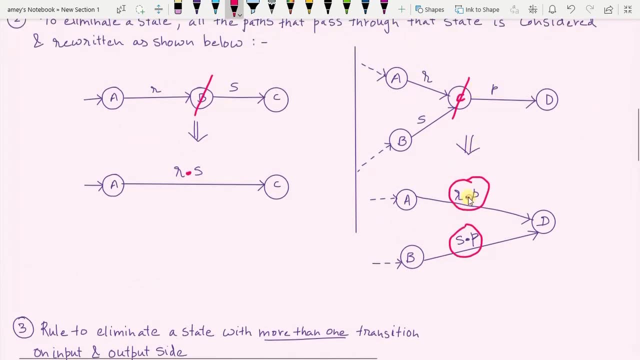 So the input that will appear will be S, dot, P. okay, this is the input. fine, why this dot is required? because it simply means that if C is not there, then A. in order to reach from A to D, what inputs are required? first, R has to be read, and after R, P has to be read only. 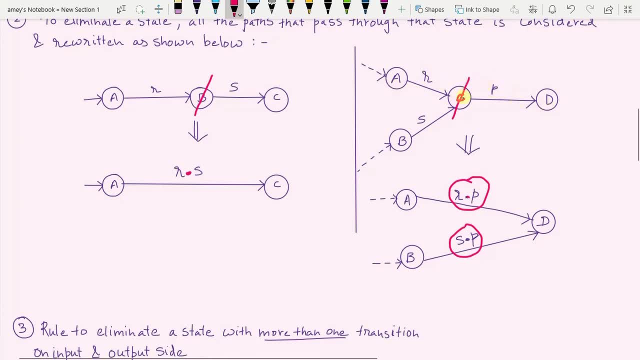 then from A you go to D. that is the meaning of it. that is why, when C is removed, you can just write the input. So the input on this direct transition, that is R, dot, P. that means first read R and then followed by P. dot means followed by P. similarly, B to C, the value is S. C to D, the value is P. 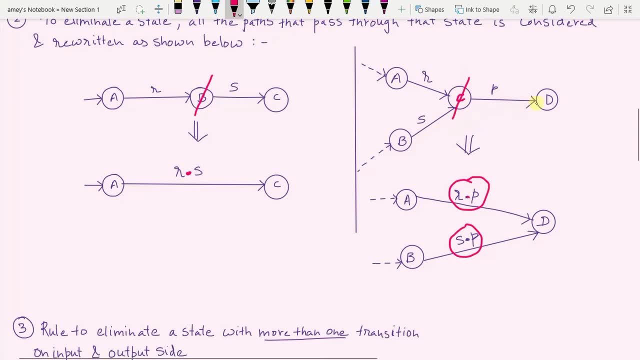 so if this is eliminated, you will have a direct transition from B to D. and what is the input that is to be read? if you want to move from B to D, first S has to be read and after S P has to be read. So it is S dot P. 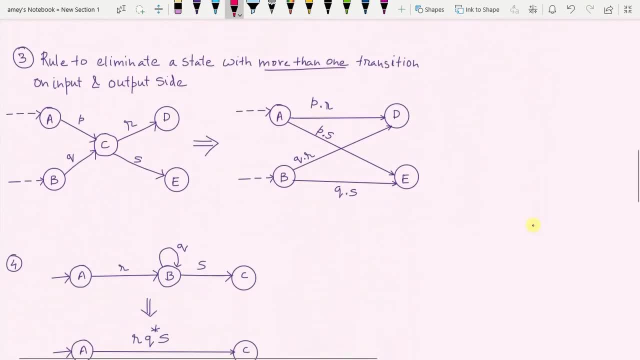 Okay, That is the meaning of it, okay. third rule: now this is slightly complicated, so what happens here is: my aim is to remove this C, but now you just see that here C is a state which has more than one transition on input and output set. okay, so that means, if I want to, 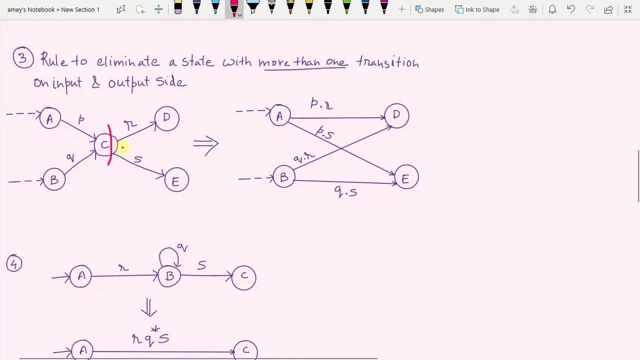 remove a state which has more than one inputs and which has more than one outputs, then what? okay, Now please note. okay, in this case, please note, if C was not there, if C was not there, then I could have said that A is, you know, directly connected to D. if C is not there. 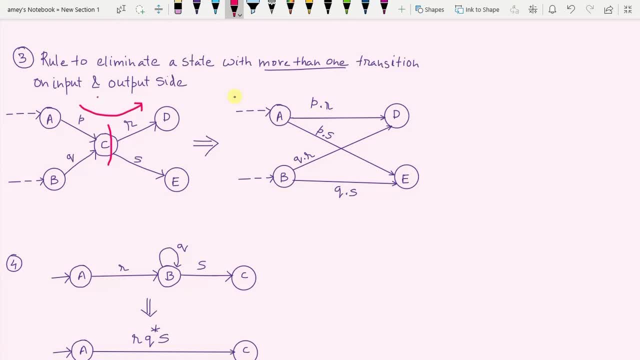 then A is directly connected to D and the input on that should be P dot R. similarly, if this C is not there, if C is not there, then B is directly connected to P and the input would be what it would be: Q dot S. and that is how I get P dot R. that is how I get Q dot. 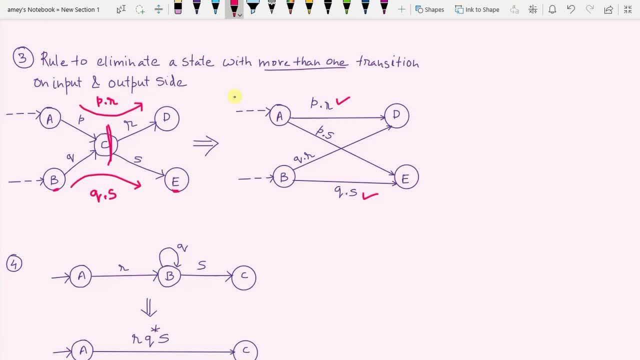 S, but also remember that you know A is indirectly connected to D through C, but A is also indirectly connected to E through C. similarly, B is indirectly connected to D through C. that is okay, but also B is indirectly connected to E through C- Okay, So you also have to be taken care of so now, since A is indirectly connected to E, if C 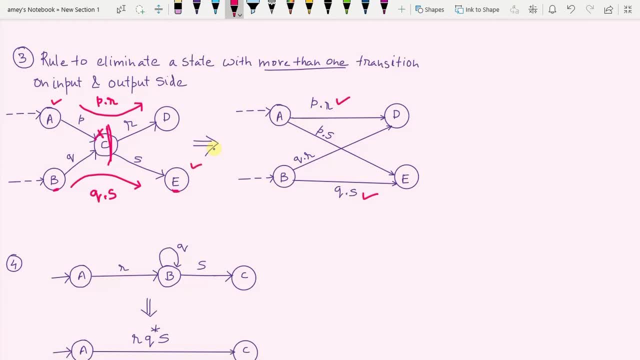 is removed. okay, if there is no C, if this state is removed, then on the transition. on the transition, do not you think you will have P dot S? okay, it is P dot S, yes, so this is that. Similarly, your B: if C is not there, then your B is not there. 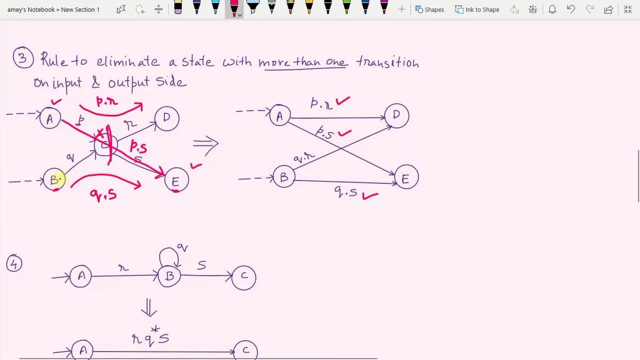 Then your B. I can say that B is indirectly connected to D. if C is not there, then B can be directly connected to D. I am sorry, and the transition that will, the input that will be appeared in here, will be Q dot R, right, So this is how the intermediate state C can be illuminated. now this rule, third rule, you. 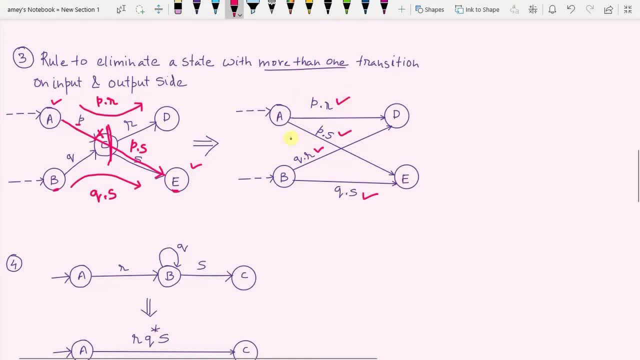 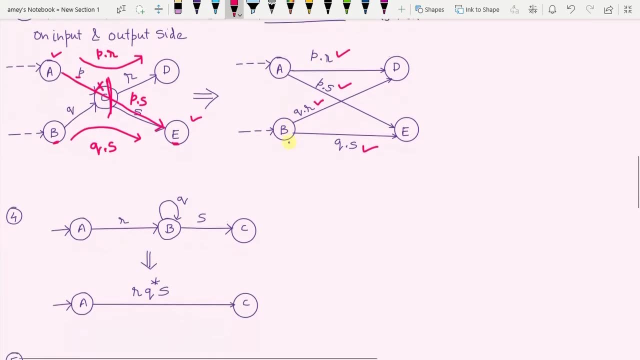 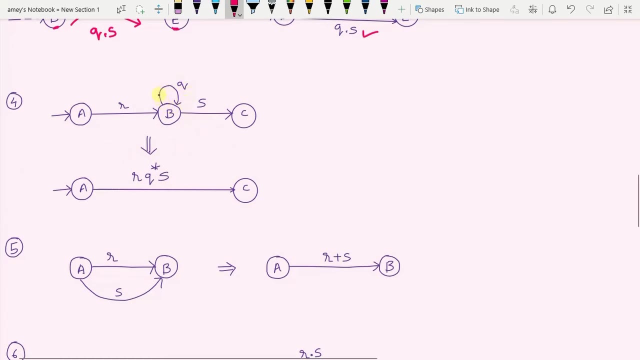 need to carefully apply: only when there are more than one intermediate state C can be eliminated. Now this rule, third rule you need to carefully apply: only when there are more than one intermediate state C can be eliminated. So this is a simple one. Next rule is very simple now, I told you, whenever there is a self loop here, it means this loop. 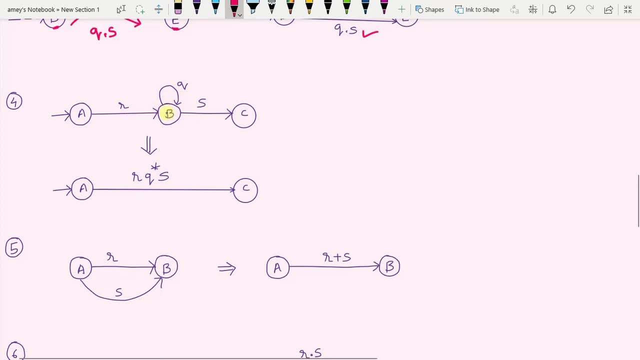 may execute or this may not execute. okay, Whenever we have self loop in automata, it simply means that this self loop is optional. we have seen this right. that means it simply means that B this transition may or may not there, and when I say may or may not be there, it simply means that the transition, the repetition, 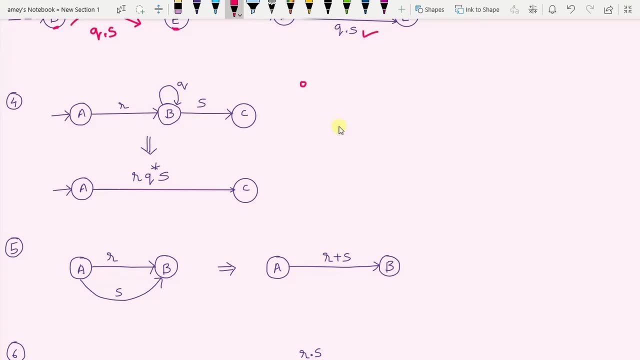 can occur 0 times. and when it occurs 0 times, it means this transition is not considered, or it can be considered n number of times, so it is 0 to infinity. so in general we have clean star right. so whenever you have this kind of condition in the automata and if you 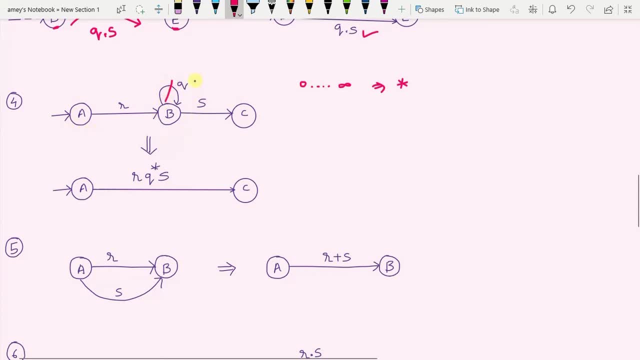 want to remove. if you want to eliminate this transition, then what you have to do, the input, that is q, you have to just write it as q raise to star, because q raise to star means what that means this q will be- will appear 0 times or more times when. q appears 0 times when. 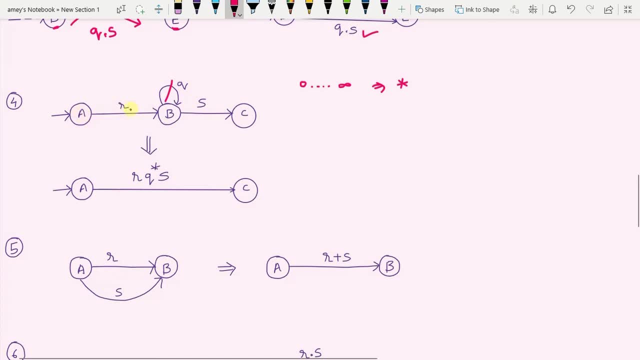 the input read. that is, from a on reading r, you can go to b, so r is read. then from b on reading s, you go to c, so c is read. So in this case, what is appropriate? From b, the self transition over here, the self loop. we have not at all considered that time. 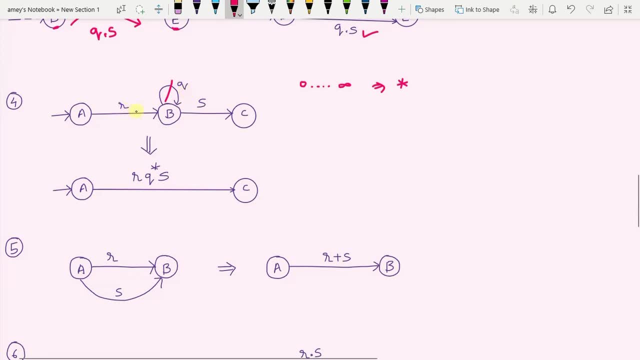 this q is 0, repeated 0 number of times. so the answer will be r dot s. but in some other instance, from a on reading r, when you go to b now, from b on reading q, multiple number of times, you may remain in b. that time q is considered. that time this q will be repeated. 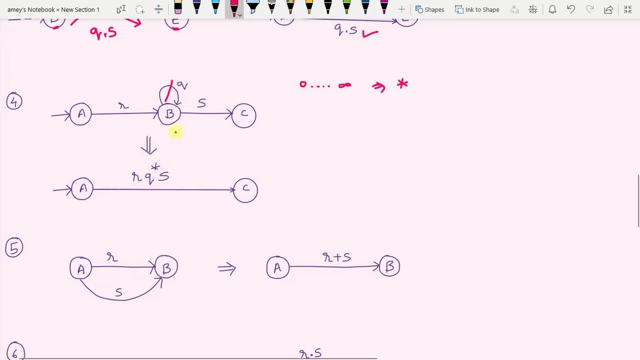 some n number of times. so in general, q raise to star. so remember one thing: whenever you want to do this, you have to do this. So remember one thing: whenever you want to do this, you have to do this. So remember one thing: when you want to eliminate self loop, you just do one thing: okay, you remove. 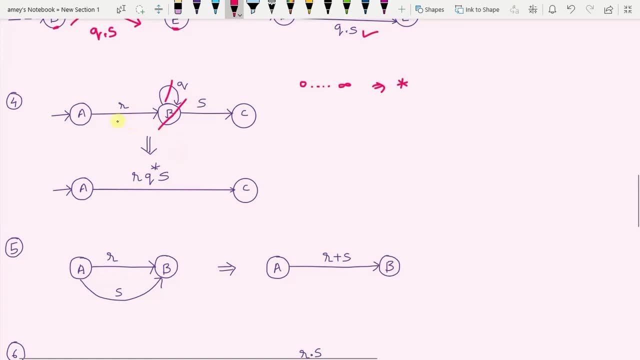 you remove the state containing this self loop and then you connect two states, this one and this one. okay, So it will be r. dot now can say: if I eliminated a state with a self loop, that self loop means what it is: the input raise to star. so that input raise to star, we write here: followed. 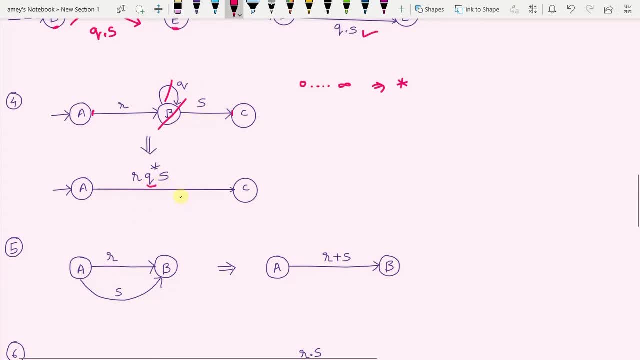 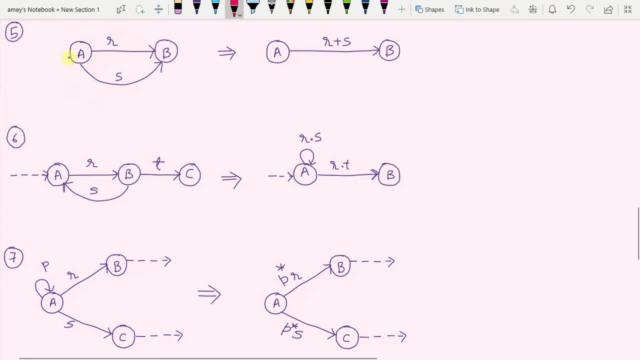 with s, okay, So the sets of outputs are respect melodies, So you keep going. Next. now, whenever you have this kind of figure, it simply means that from state A, on reading R, you go to B, or second base, from A, suppose, you read S, then also you go to B, So that 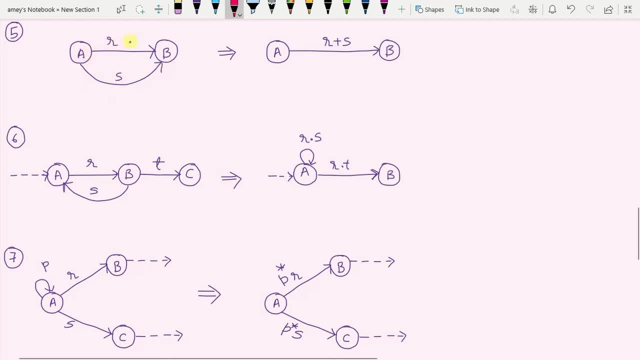 means from A. either when you read R, you go to B, or when you read S, you go to B. So there is OR, and OR means plus. So if you want to eliminate these two transitions and make it as one transition, Okay, see, both the transitions are going to B. 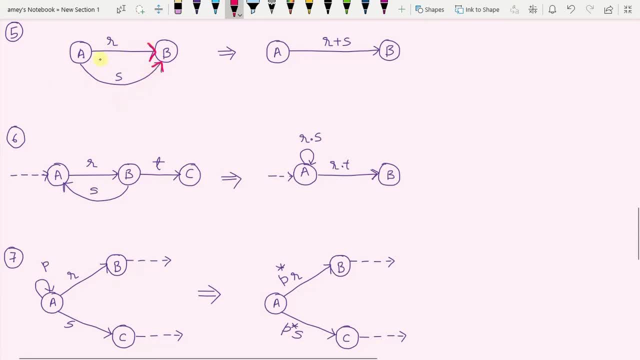 Right. so when you want to eliminate this and make it as one transition, you can just draw a single transition line. So it simply means that from A, either by reading R you can go to B, or by reading S you go to B. OR means plus. Okay, that is the meaning of it. 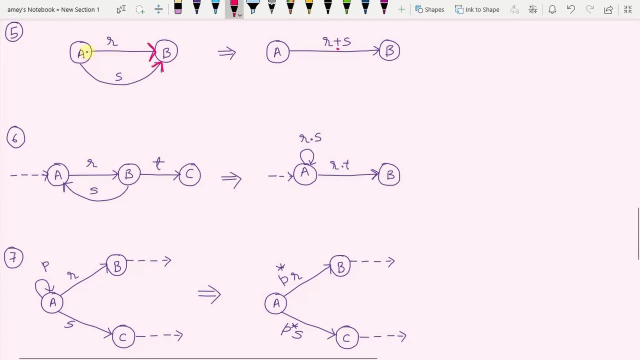 Now the meaning would have been have been different if this was a loop. that means if from A it was going to be, and from B if it is coming back to A, so from A you are coming back to A. if that was a case, then it is this rule will not be applicable. then that is called as loop, which we are going. 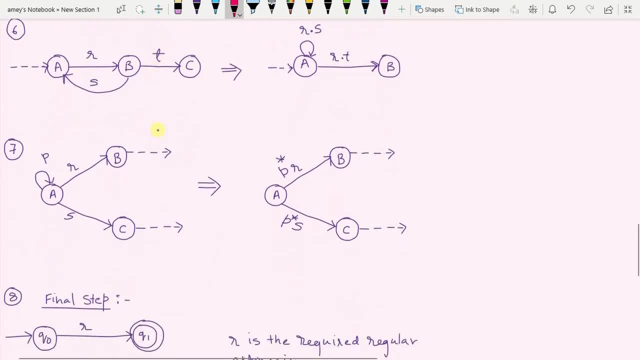 to see next Now here, now see, I was just talking about this particular thing. just see, I begin with state A. from A on reading R, you go to B, and from B on reading S, you come back to A. so this is basically a loop: you start from A, you come back to A. now, if you want to remove, 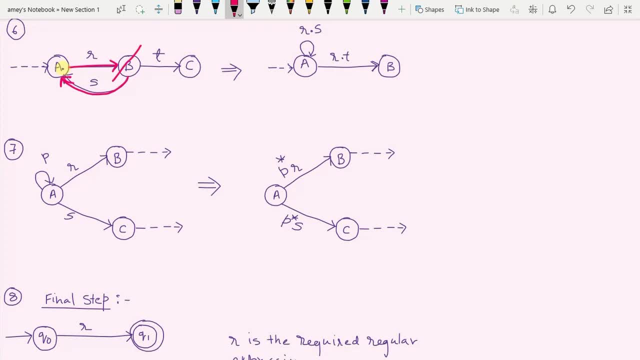 this loop. that means, if you want to eliminate this B, what will happen now? you will have to see two things. one: okay, first you ignore that there is a. there is this transition. okay, ignore that. there is this transition, that is transition from B to A. suppose this was. 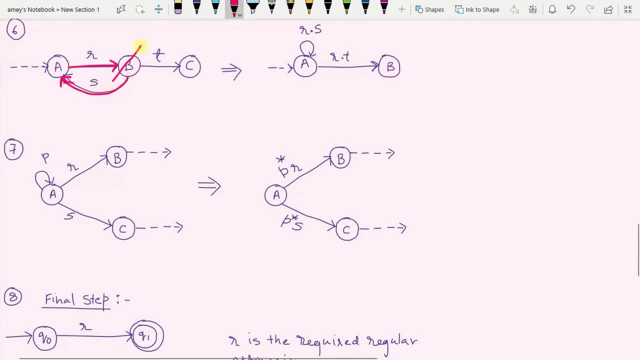 not there, Then It simply means that if I eliminate B, I will have to directly connect A and C with one transition, and the input will be read as R dot T. okay, so that is why I have written here R dot T and I have a direct transition from A to B. but now there is also second thing. 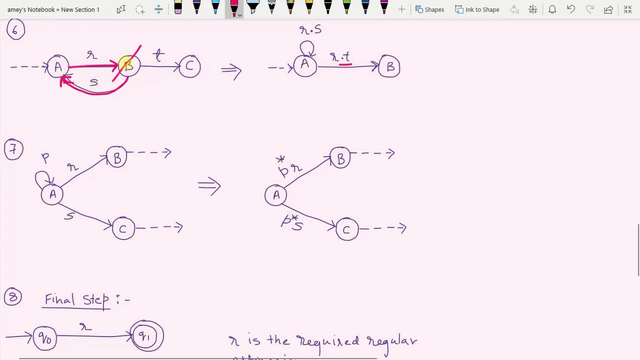 that you need to see: from A on reading R, you go to B, and then from B on reading S, you go to A. so there is a loop involved here. so when you eliminate this B, There will be also an impact on this particular loop. okay, the impact on the transition from: 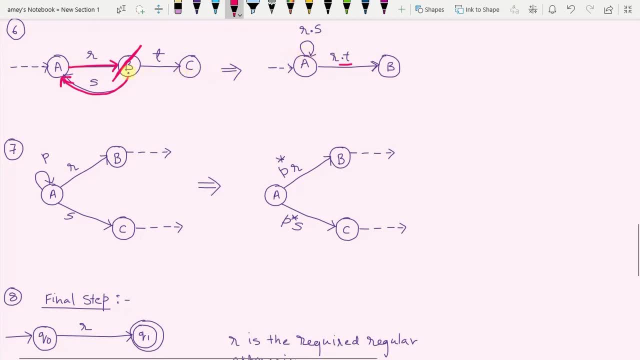 A to C. we have already seen, but there will be also another impact from a transition for a transition from A to A itself. so when B is removed, this can be written as you can write this as a self loop over A. okay, you can write this as a self loop over A and this. 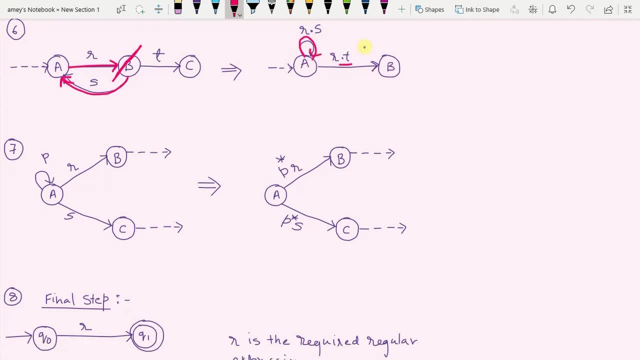 can be written as: So this is the loop. So this is the loop simply means from A on, first on reading R and followed by S. So from A, okay, it simply means from A when R is read and then followed by S when I say, followed by, it is dot. So 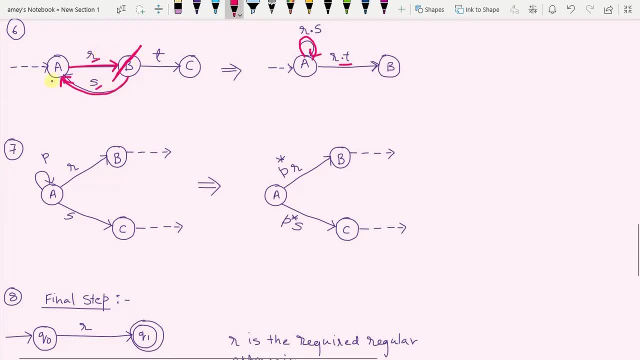 when R is read and next after R, when S is read, then you come back to A From A. when R dot S is read, you come back to A. So what you can do is you can then remove B, okay, and you can just introduce a self loop over A and write R dot S. So please note there. 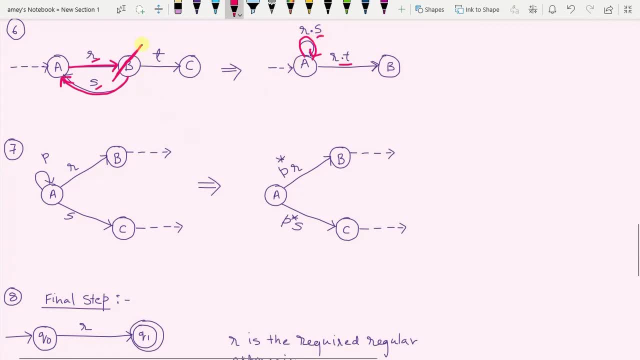 are two changes that are going to happen, Since B is connected to two things: B connects A to C and B also connects A to itself. So in the first case- connecting A to C- when B is removed, you will have a direct transition from A to C and input will be R dot T You. 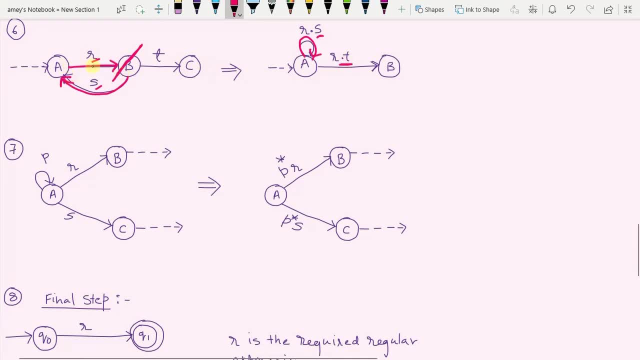 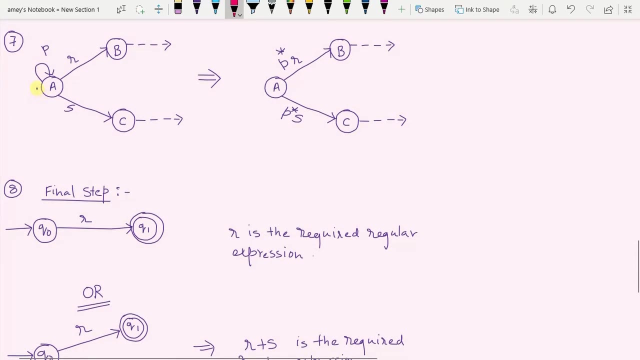 have seen already Now, when you consider R dot S, you will have a direct transition from A to C and input will be from A to A itself. When B is removed, then you will have- you will see- a self loop over A with R dot S. okay, Next, Now I continue with the same thing. Now, for example, you have 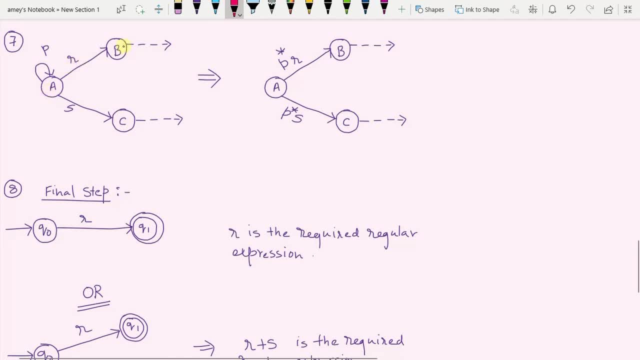 this state: A: okay. From A on reading R, you go to B. From A on reading S, you go to C, and A has a self loop over A. Now, many a times, if you want to remove this self loop, I told you what is the meaning of self loop. 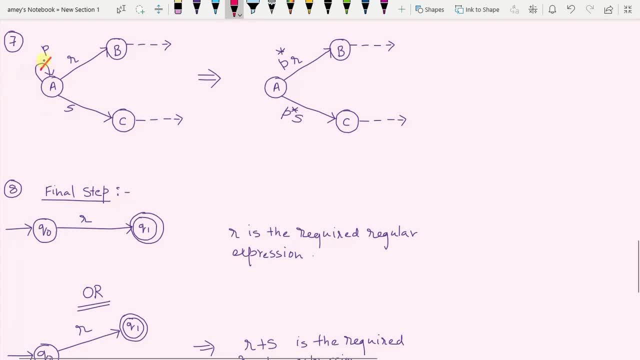 Self loop only means zero or more times. So the input which is there on the self loop input, you have to write it as input- raise to star. But this self loop also has impact on B. It simply means that from A on reading P, zero or more times, followed by R, exactly. 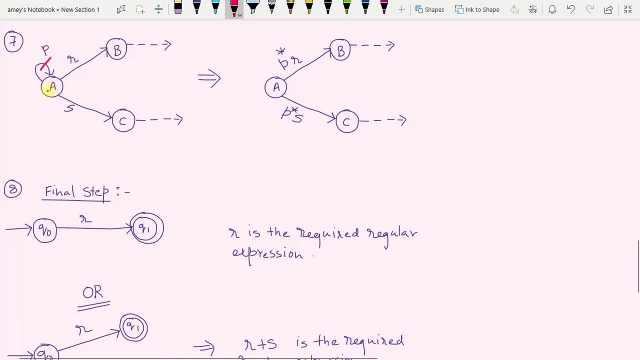 once you reach B, Similarly from A on reading P zero or more times, followed by S, then you go to C. So when this self loop is removed, the transition that connects A to B, that is, this transition, will have P star B, where P star means P is repeated 0 number. 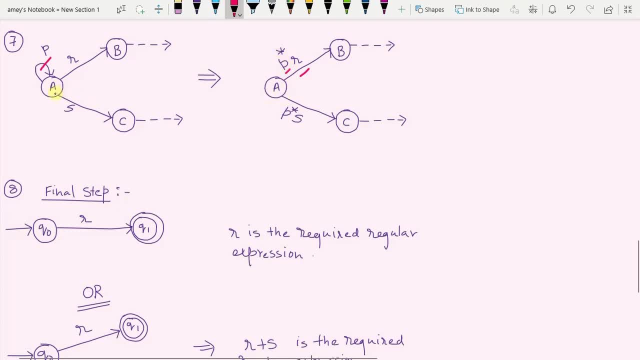 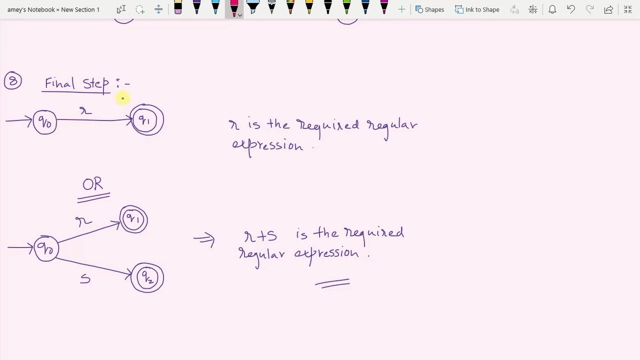 of times, or infinite number of times. Similarly, the transition between A and C can be then written as P star S. So the last thing now, the final step. Now, after following all these steps, after doing this elimination as and when required, you will finally reach a state. 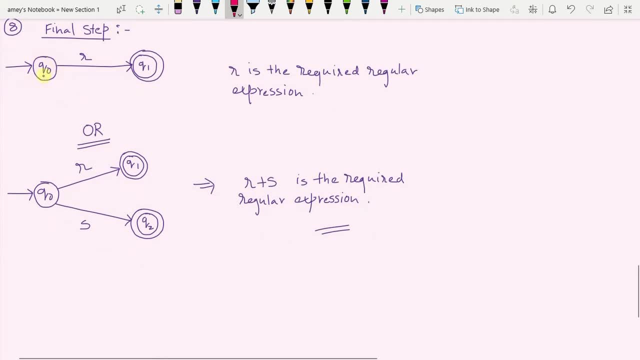 wherein you will have a single input state or its single start state and you will have a single final state. Then whatever regular expression that you are going to obtain on this transition line, that regular expression is the required regular expression for the automata that is given. Many a times a finite automata can have. 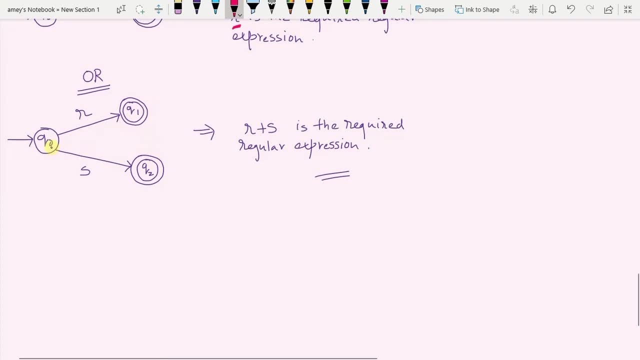 more than one state. So you may come to this situation wherein initial state is connected to one output and initial state is also connected to the second output, and you will have two regular expressions appearing on both the transition lines connecting initial and the final state, both the final states. So in that case the final regular expression will be: 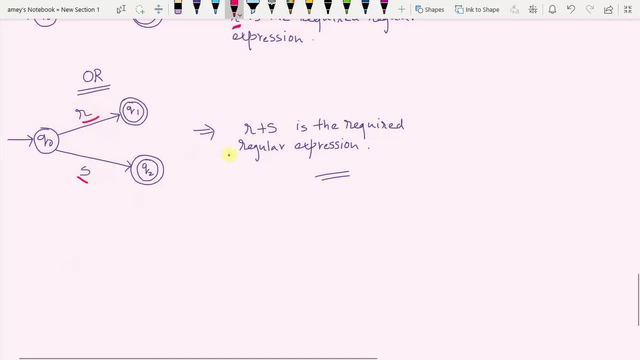 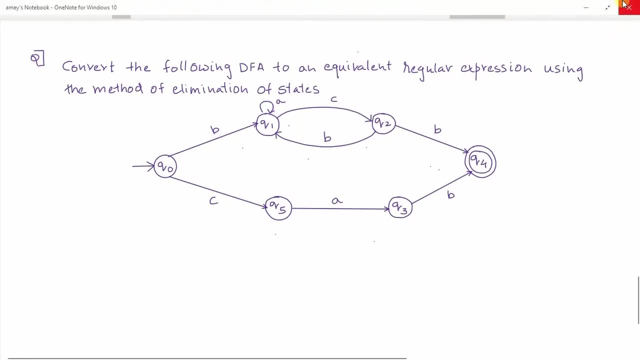 either R only or S only, and so on. So the regular expression can be written- final state Only- as R plus S. Now this is a problem that is given to us and we are supposed to convert this particular finite automata to a regular expression. So how shall we begin? Let us 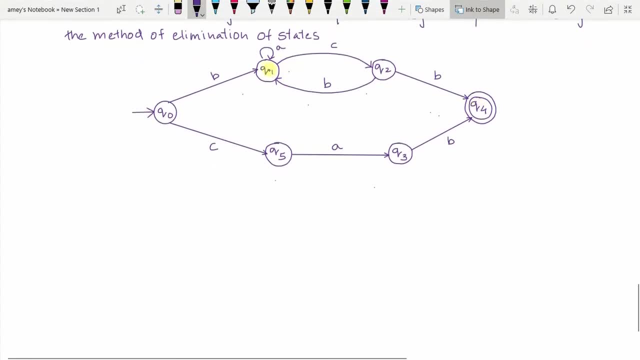 start analyzing different states. Now you see here one thing is very clear: See, from Q naught on reading C, you go to Q phi. From Q phi on reading A, you go to Q phi on reading A, you go to Q3. and then from Q3 on reading B, you go to Q4. There is a straight and direct. 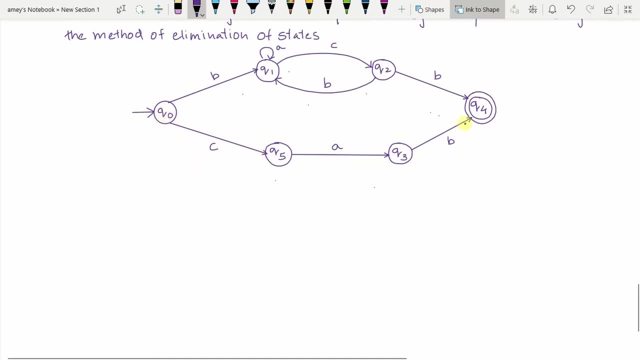 link that is connected, connecting Q naught and Q4, and this link it goes through two states, that is, Q, phi and Q3.. So if I eliminate these two states then there will be a direct link that can go from Q naught to Q4 and that. So I will just write. 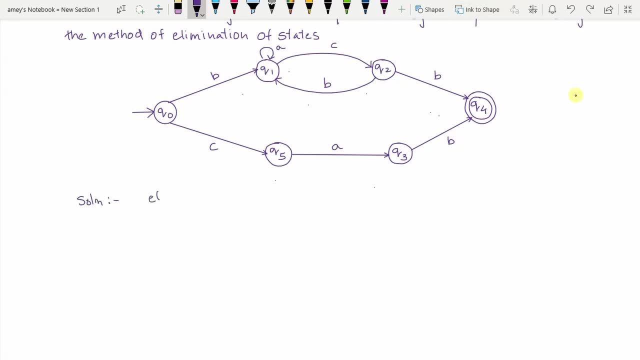 Okay, States Q5 and Q3 we get. So you will have state Q naught. Okay, You will have state Q naught And then, And then Q naught to Q4. you can show a direct link From Q naught to Q4. you can show a direct. 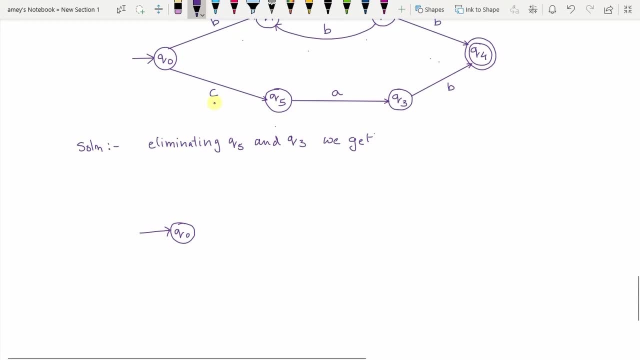 link and the string that is read on it will be CAB. So you have Q4 here, which is a final state, And from Q naught to Q4 you can show a direct link, CAB. So what we have done, The intermediate states Q5 and Q3. they are eliminated, so there is a. 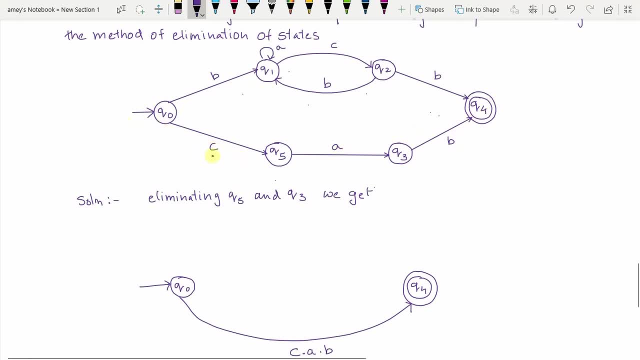 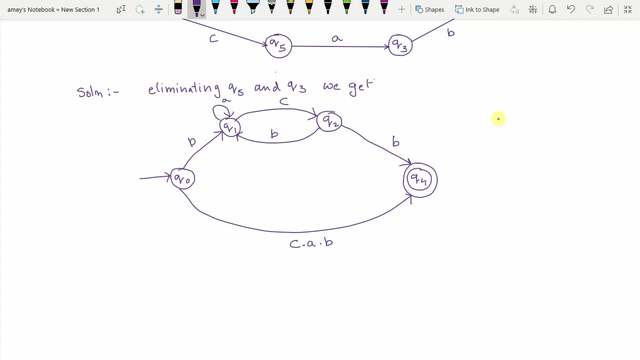 direct link connecting Q naught and Q4 and the direct link is CA and B. We have not analyzed the top part, so top part will write as it is will down to Q4.. So this is what we get. Now look see what happens is we have already seen a property and that is this property. 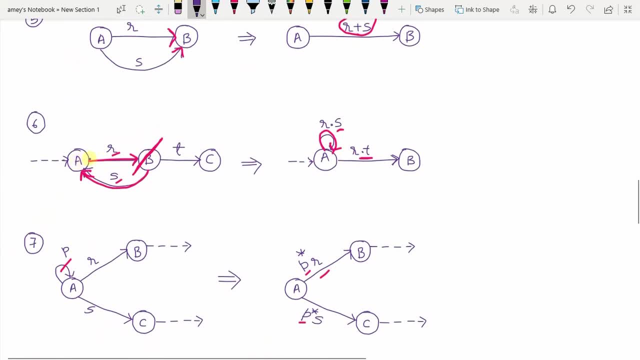 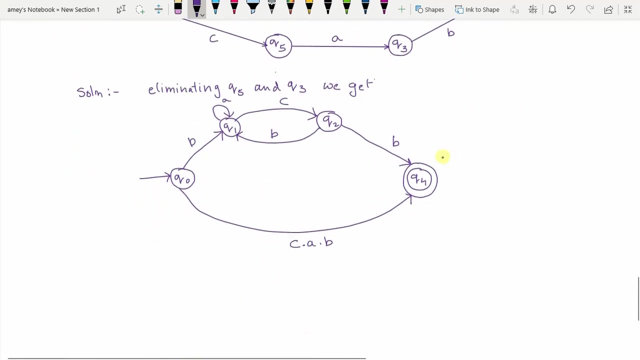 Okay, So from any state, if there is a on reading a particular symbol, you go to another state and then from that state on reading another symbol, if you come back to the same state, then eliminating this b. okay, it would simply mean that there is a self to power a with rs. okay, so we are going to use the same mechanism here. 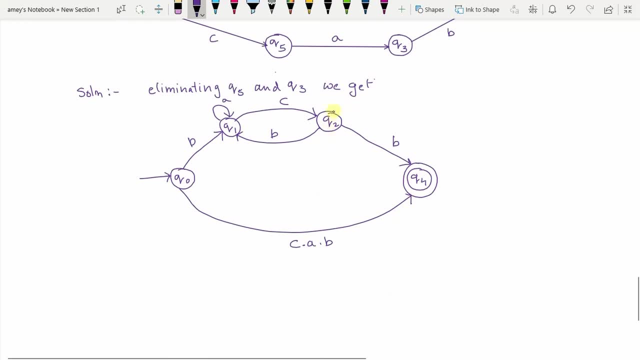 I will try to eliminate this q2. now q1 is connected to q4 through q2. so if this q2 is removed, one thing will be: from q1 there will be a direct link going to q4 and the string that will be read on it will be cb. okay, that is first thing. okay, so if I remove q2, if I remove this q2, two things will happen. one, there will be a direct link going from q1 to q2.. 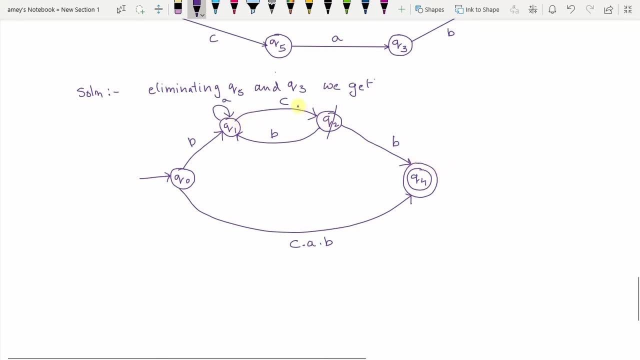 And the string or the regular expression that will be reading on top of it will be cb. but q2 is also associated with this loop here and it is a self loop. so when q2 is removed, you will see that there is a self loop that you are going to get on q1 and the self loop will have input that is cb. okay, so. 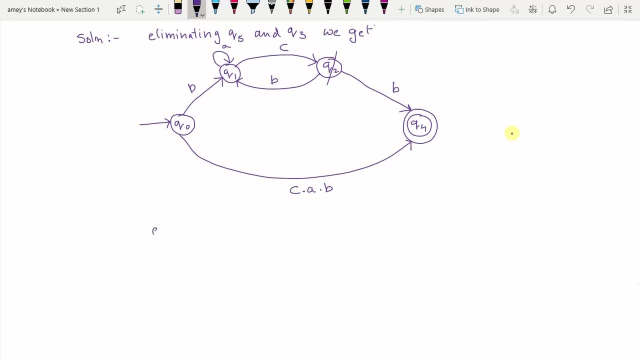 So eliminating, eliminating state q2, q2- we get. okay, first of all I will write q0 as it is, Then. Then this is q4, state q4. q0 will be connected to q4 with cab as the input. now we are eliminating q2, so what we will have is: we will have state q1. okay, so we will have state q1. then q0 will be connected to q1. 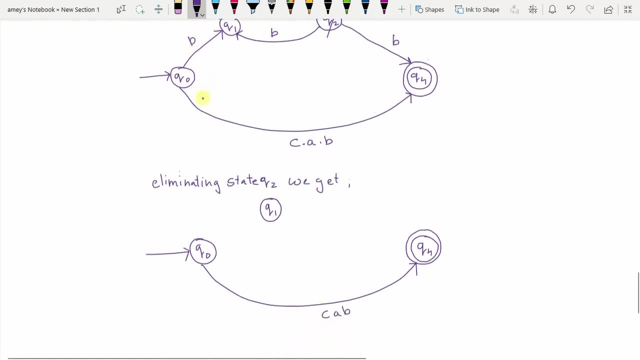 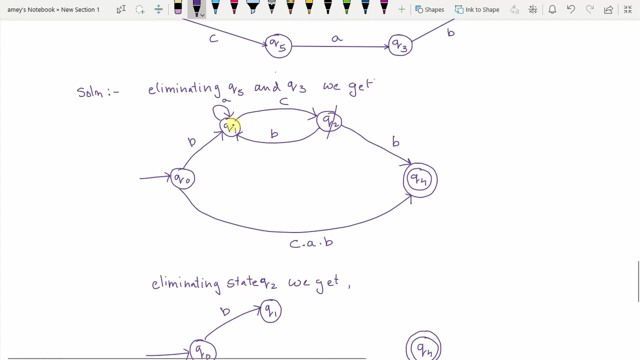 Then Then state q1 through b, so there is no change. so I will write this as it is: q0 will be connected to q1 through b. then, as I told you, when q2 is eliminated, there will be a direct path from q1 to q4 and the input that is read will be cb. so when q2 is eliminated, as I told you, there will be a direct path from q1 to q4. there will be a direct path from q1 to q4 and the input that is read will be cb. so when q2 is eliminated, as I told you, there will be a direct path from q1 to q4. there will be a direct path from q1 to q4 and the input that is read will be cb. so when q2 is eliminated, as I told you, there will be a direct path from q1 to q4 and the input that is read will be cb. so when q2 is eliminated, as I told you, there will be a direct path from q1 to q4 and the input that is read will be cb. so when q 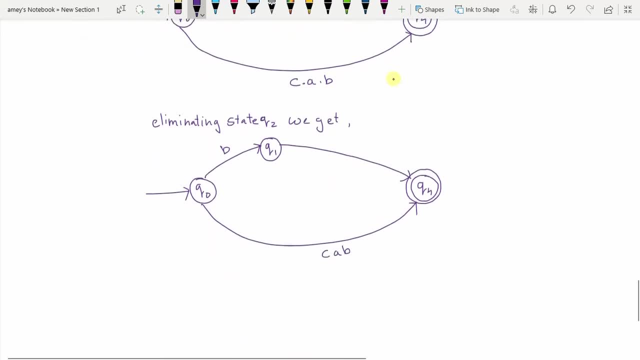 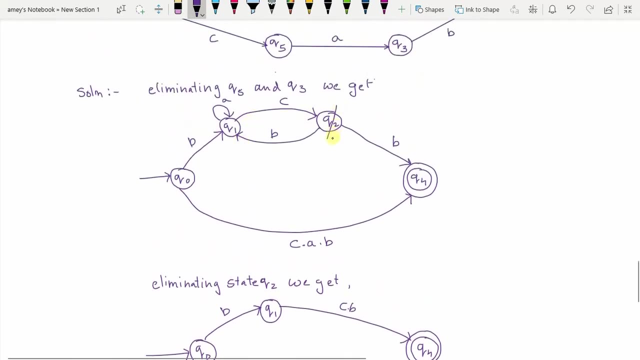 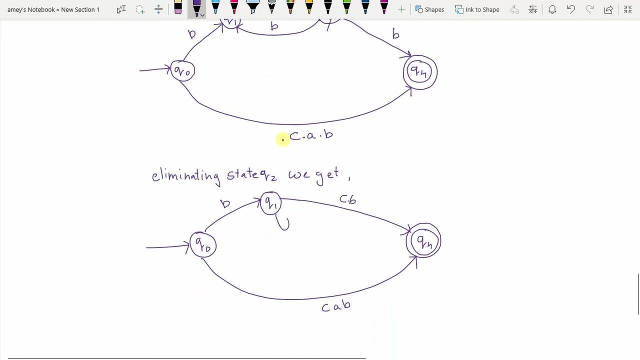 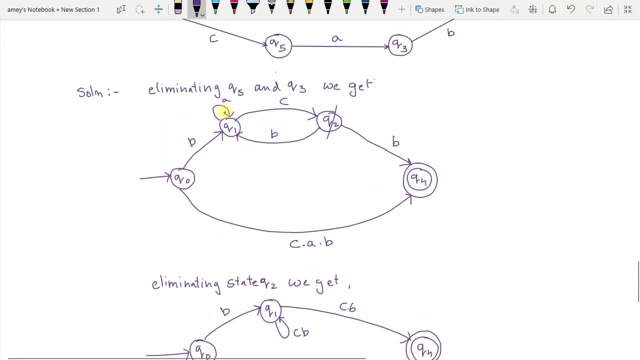 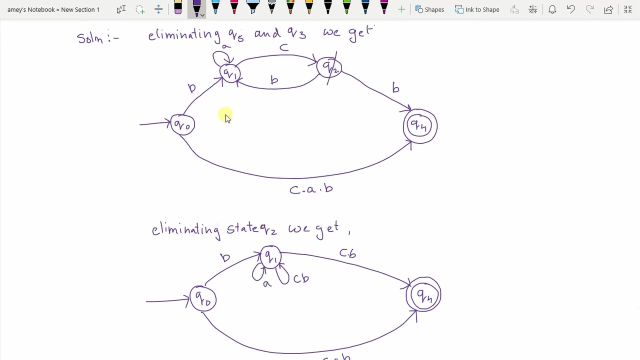 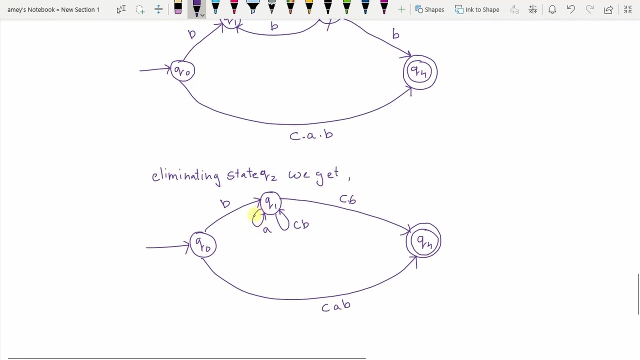 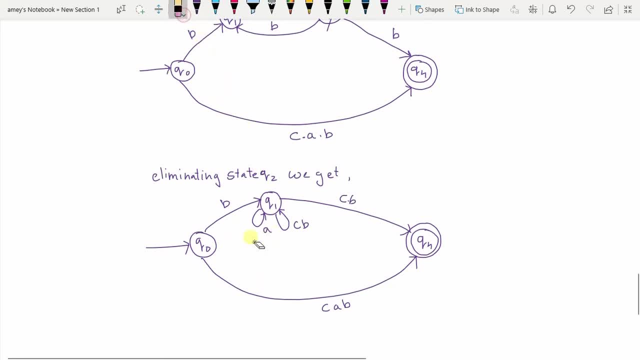 when q2 is eliminated, as I told you, there will be a direct path from q1 to q4 and the input that is read will be cb. I will remove one self loop and I can write this as a or cb. a That means whether it. 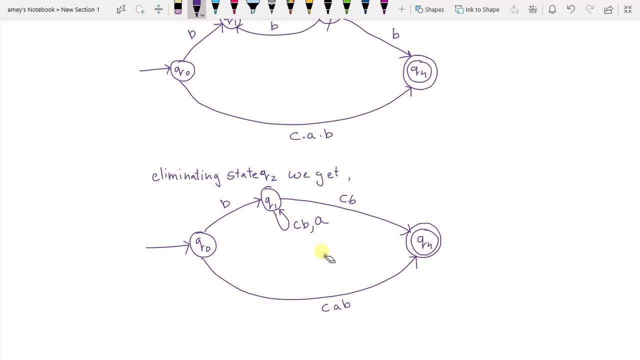 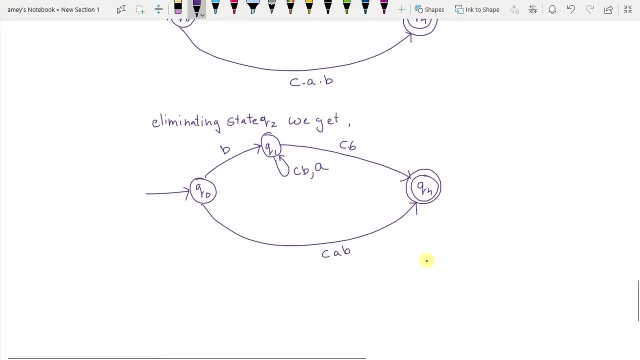 is cb or whether it is a, from q1. on reading any one of these, you go to q1 itself. So this is what we are getting so far. Next, what I will do, looking at this figure, what I can figure out is: okay, I will try to remove this self loop. Removing a self loop there. 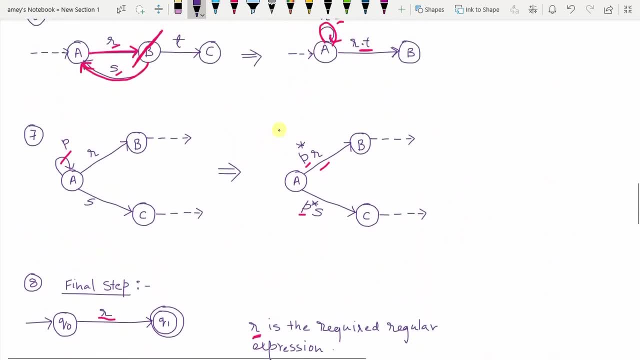 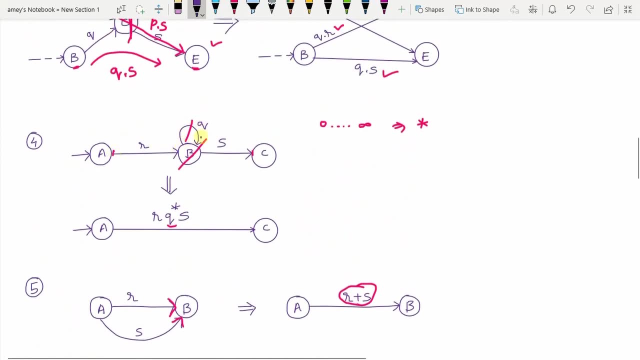 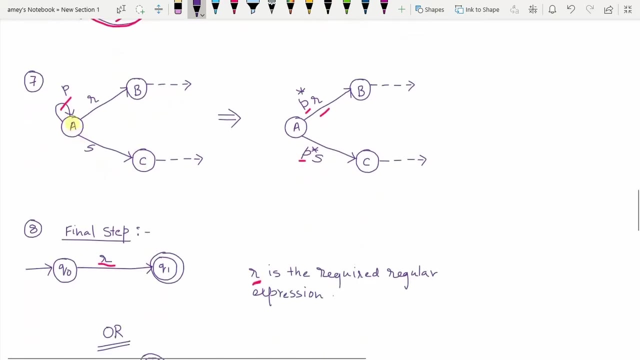 is a rule that we have already seen. Okay, You see here. okay, here, When you remove a self loop, the input over it can be written as that input is to star. Similarly here see: when the self loop is removed, p becomes p star And of course it is associated with. 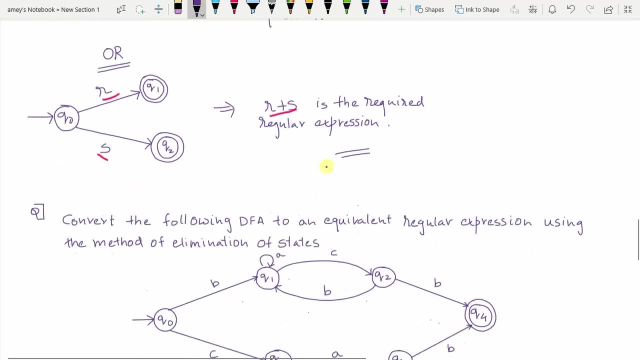 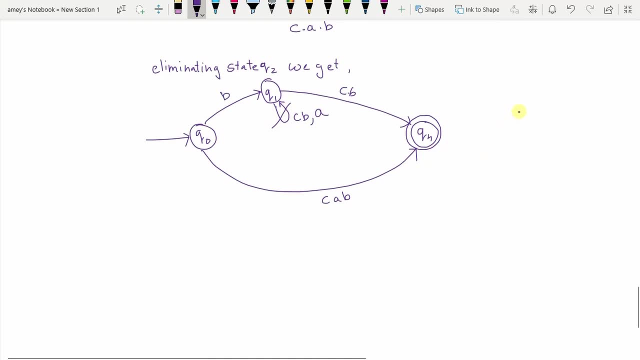 others, so it will be reflected in other transitions Over here. over here, okay. when self loop is removed. okay, I will just tell you self loop is removed. it will be written as a cb raise to star, Okay. 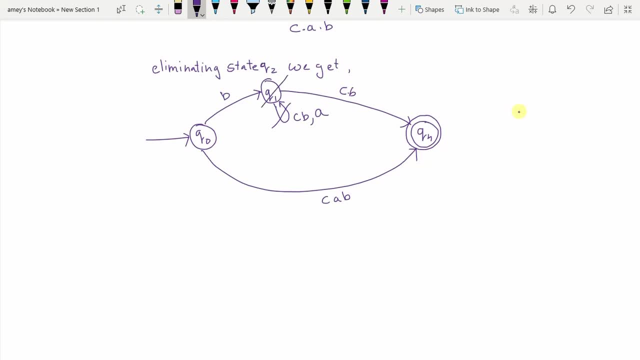 Further. if I am going to remove this, then there will be a direct path connecting q0 and q4.. If I remove this q1 itself, there will be a direct path connecting q0 and q4 and it will be read as b. Then, since this self loop is removed, this input will be read as: 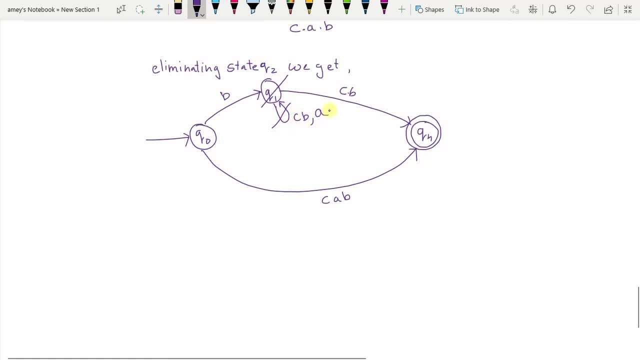 cb, comma a or cb plus a, the whole star and cb. Okay. So eliminating the self loop, Okay. Eliminating self loop over q1 and then q1 itself, we get okay. So in-between two separations, right. 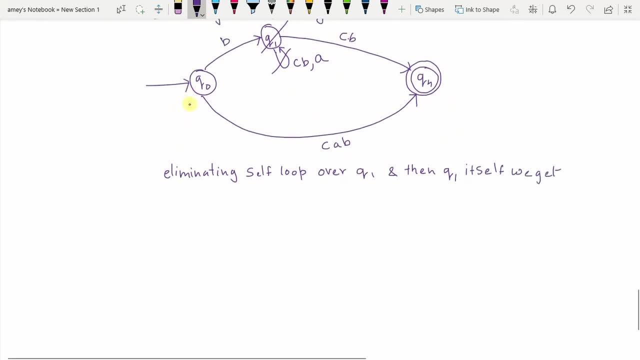 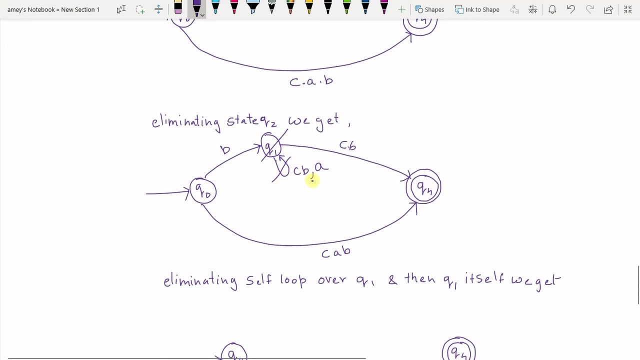 Okay, Now what we are going to get: Q0, that is a start state, and Q4, that is a final state. Fine, Now, from this side, Q0 and Q4 will be connected through CAB. That is okay. Now, when this self loop is removed, this term over here. okay, this will be read as CBA. Also, I told you that whenever there is comma, there is a rule. See the very first rule that we have seen. 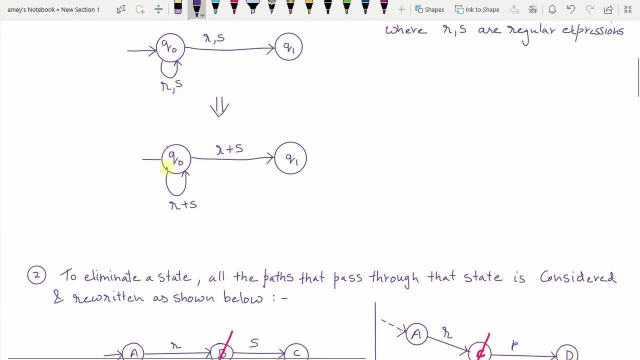 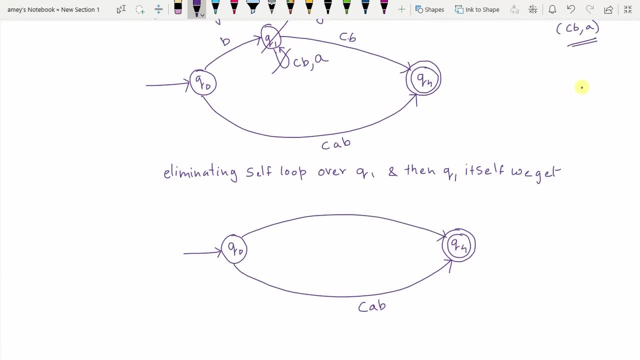 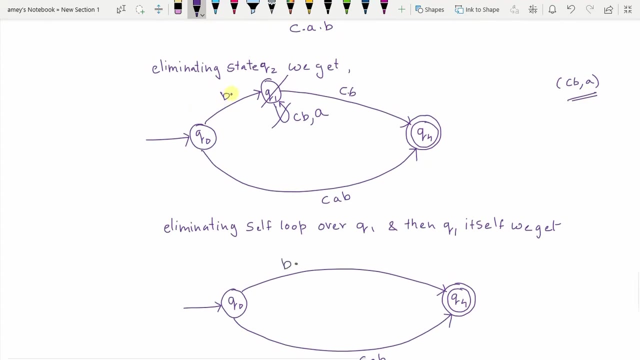 What the rule says. If there is a comma, then comma can be replaced with plus. There will be a direct transition from C to A, Q0 to Q4.. How B will be read, followed by: now: there is a self loop here, right. So when self loop is removed, the entire term over here will be raised to star.